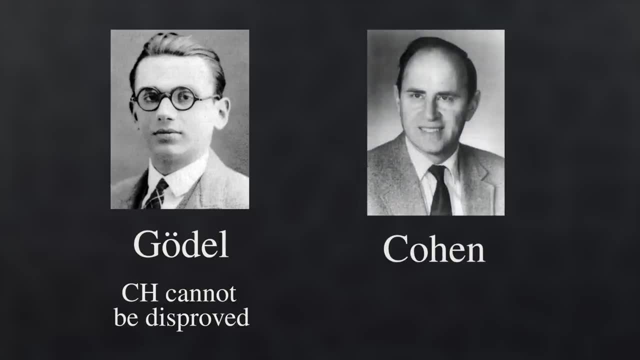 purely from the axioms. And in 1963, Paul Cohen showed that the Continuum Hypothesis is not inconsistent with the axioms of set theory, so it can't be proved from the axioms. A single nugget will have changed the axioms of set theoryarts. 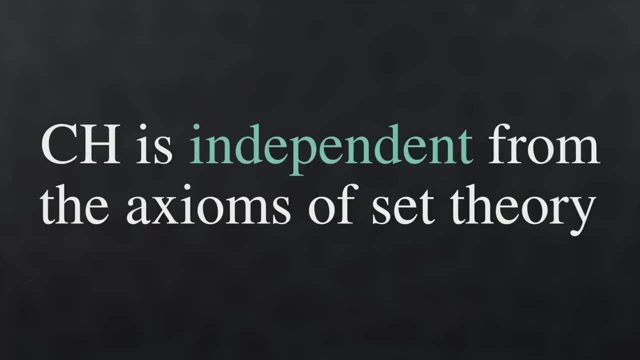 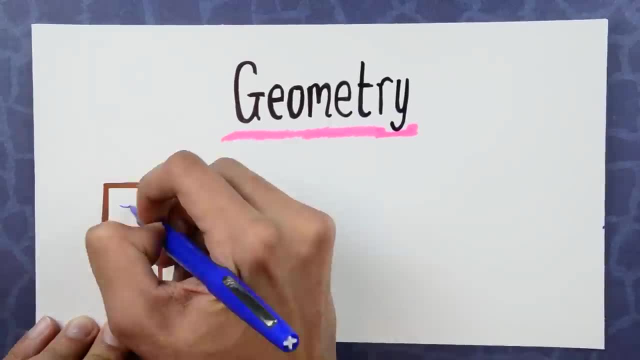 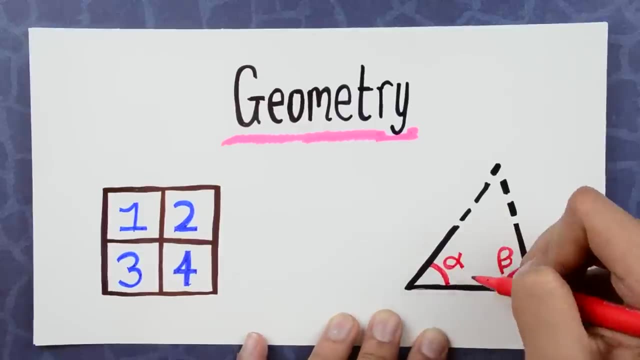 We say that the continuum hypothesis, therefore, is independent from the axioms of set theory. This notion may be familiar from geometry. When creating the Foundations of Geometry, Euclid laid out four axioms that geometry should always satisfy, But then he laid out a 5th axiom, the so-called parallel postulate. 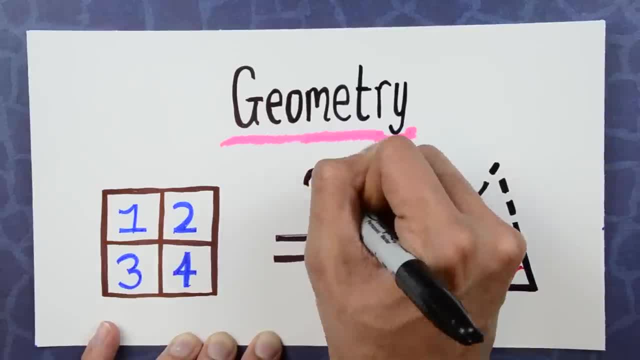 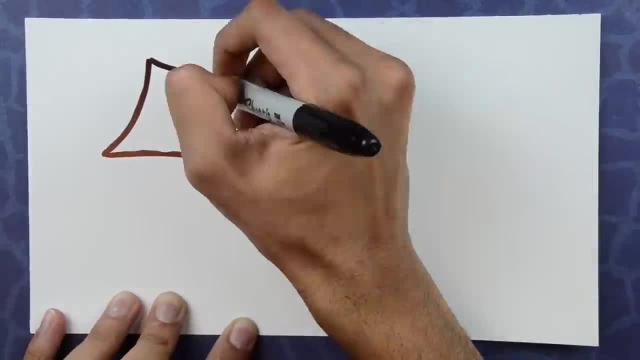 The question was: could you prove or disprove the parallel postulate purely from the previous four axioms? Well, if you consider plane geometry, then the parallel postulate is true, along with the other four axioms. so there's no way to disprove. 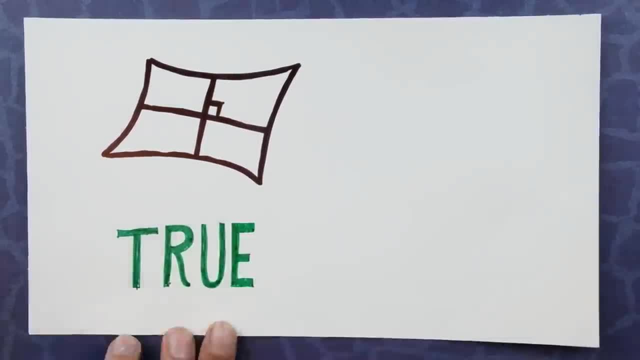 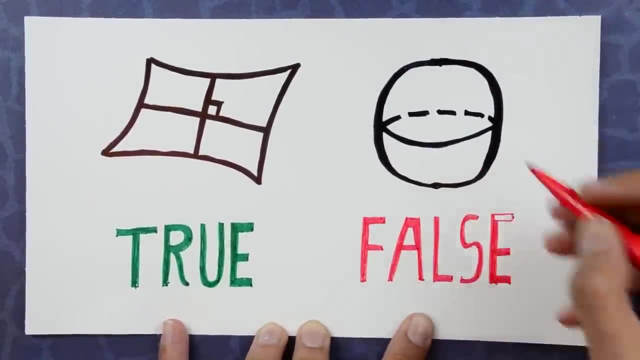 the parallel postulate because there's an example of where it's true. However, if you consider spherical geometry, then the parallel postulate is false. so there's no way to prove the parallel postulate because there's an example of where it's false. So it doesn't make sense to ask. 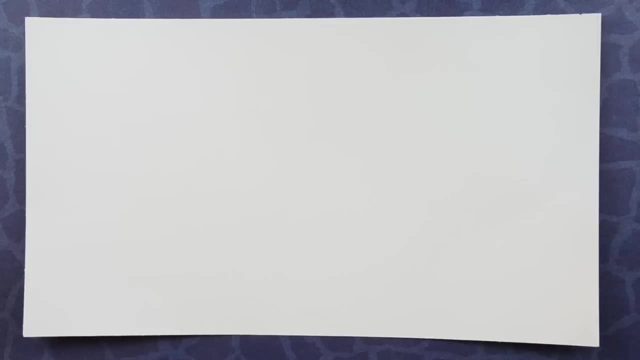 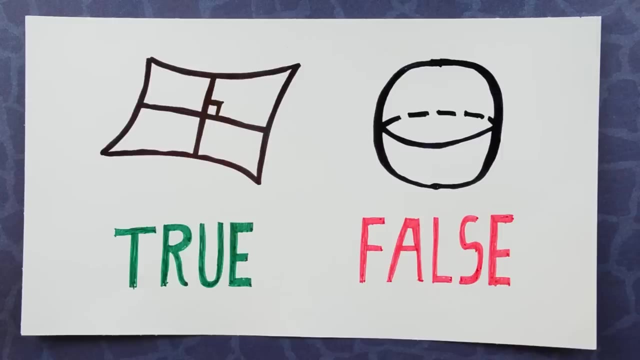 is the parallel postulate true or not? The answer is: if you want it to be true, there's a universe where it's true, and if you want it to be false, there's a universe where it's false. A similar phenomenon occurs with the continuum hypothesis: There's a universe where it's true and there's a. 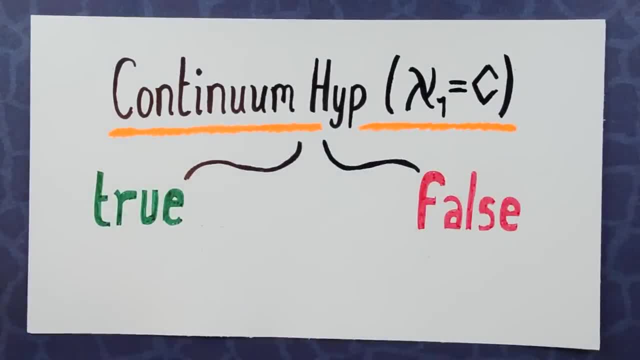 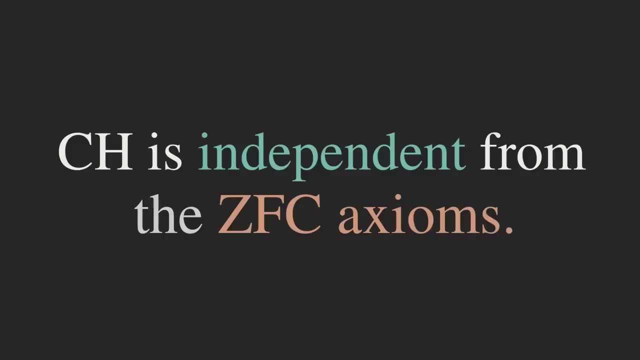 universe where it's false. So now let's be precise. When we say axioms of set theory, what do we mean exactly? We mean the so-called ZFC axioms of set theory. ZF stands for Zermelo and Frankel. 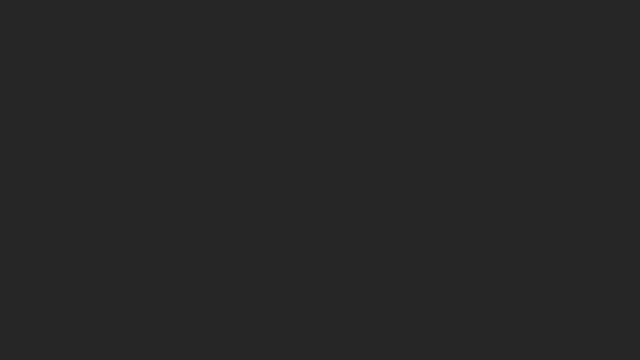 who are two mathematicians working in set theory. For example, it includes the axioms of set theory of the empty set, which simply says that there exists an empty set, or the axiom of the power set, which says that every set has a power set, ie a set that contains all subsets of that set. 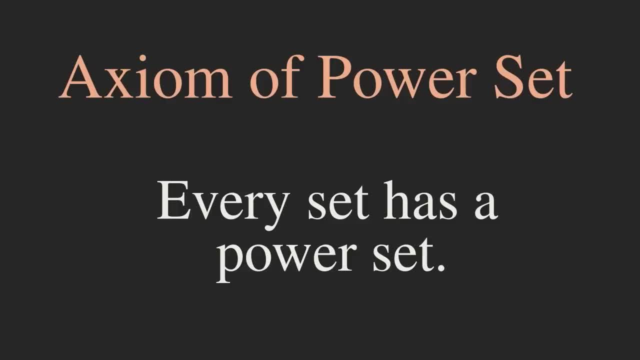 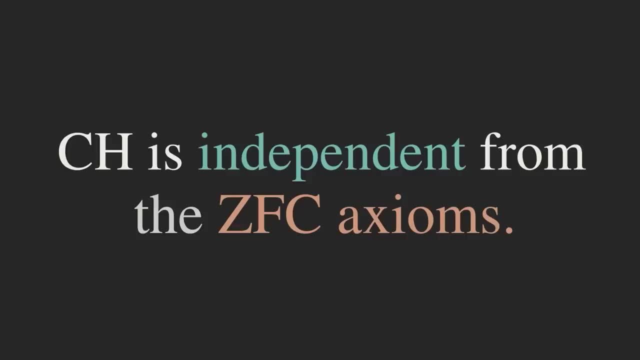 The point is, these axioms are things that you would reasonably expect to be true as a starting point for math. So to prove that the continuum hypothesis is independent of the ZFC axioms, we have to provide a universe satisfying these axioms, where the continuum hypothesis is true. 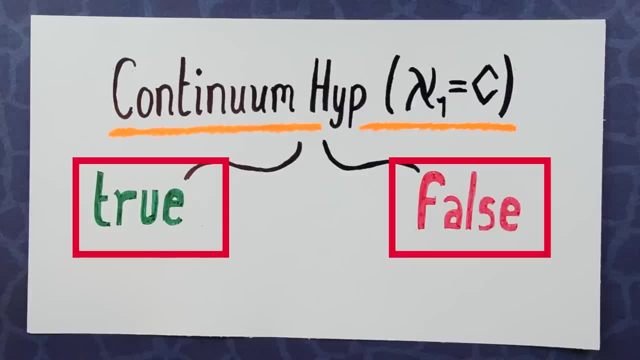 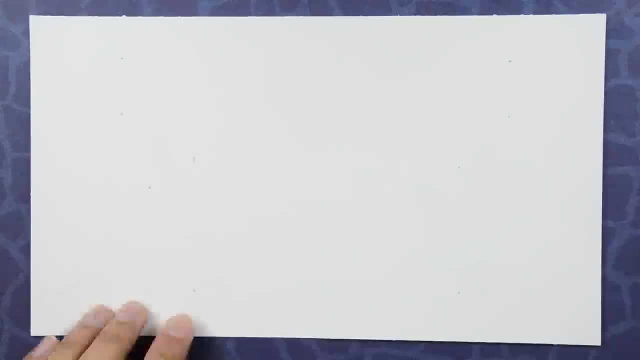 and another universe satisfying these axioms where the continuum hypothesis is false. The precise word for universe in set theory is model. A model of ZFC is a pair, m- epsilon, where m is a set and epsilon is the belongs to relation. All of the axioms of ZFC have to be: 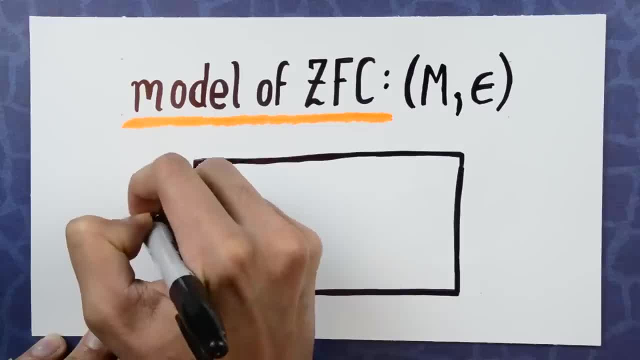 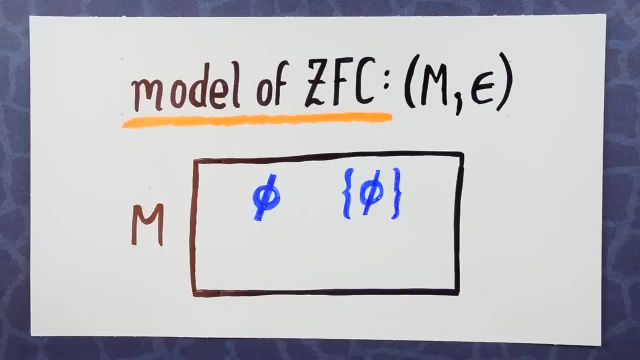 true for elements of m. For example, in a model m of ZFC there has to be an empty set in m by the axiom. The power set of the empty set is in m by the power set axiom. Not only is constructing a model of ZFC hard, it's actually, strictly speaking, impossible. 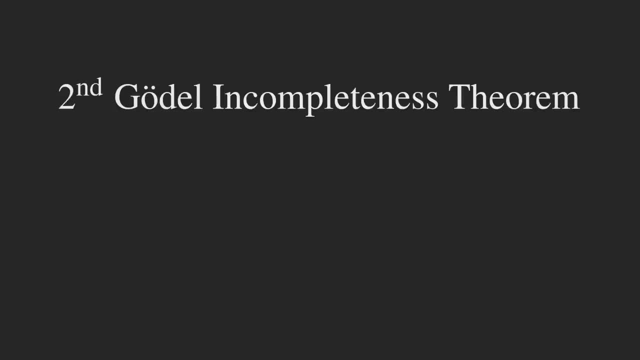 In the 1930s, Gettle published a set of theorems called the Gettle incompleteness theorems. The second of these theorems implies that you cannot construct a model of ZFC while working in ZFC. So our original plan of constructing a model of ZFC, where the continuum hypothesis was either 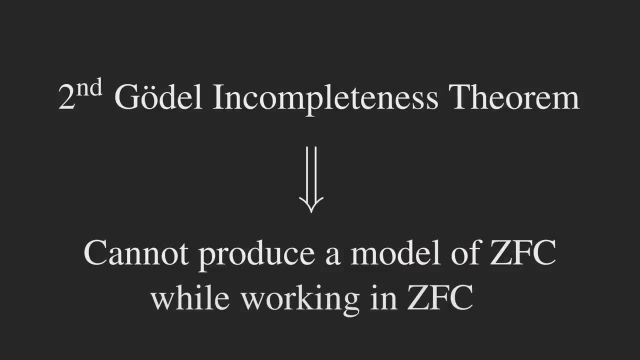 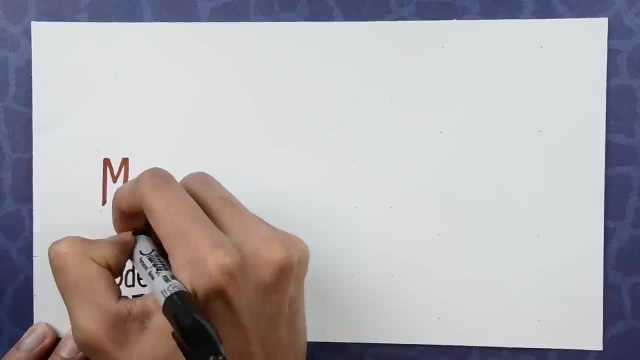 true or false won't work, because you can't even construct a model of ZFC with the correct Mutta logs for the 선생님. So the correct statement is the following: We first need to assume that we are given a model of ZFC. say m. 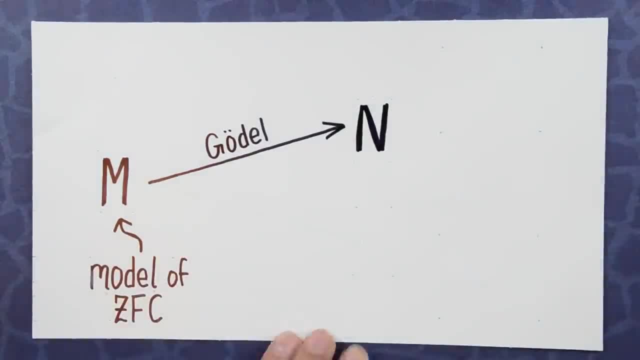 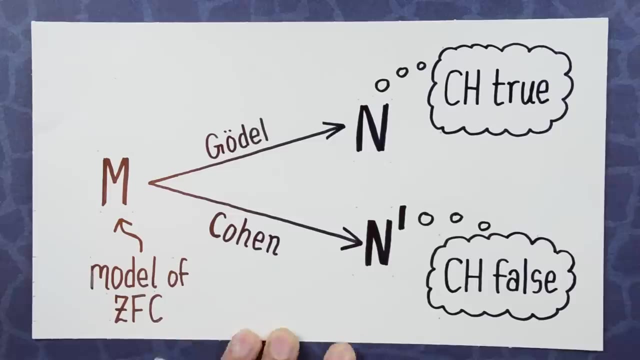 Gettle then used m to construct a model n of ZFC where the continuum hypothesis is true. Cohen used m to construct a model n´of ZFC where the continuum hypothesis is false. How is Gettle's proof? They actually aren't bimath를ies. 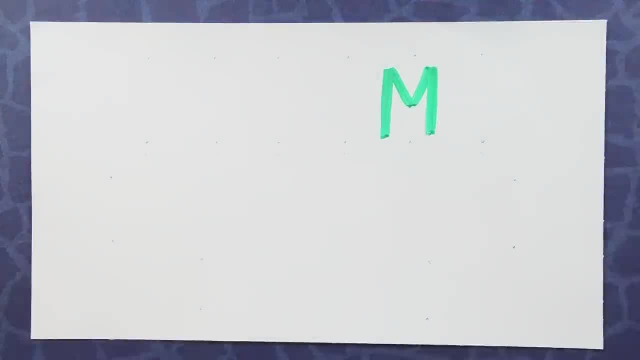 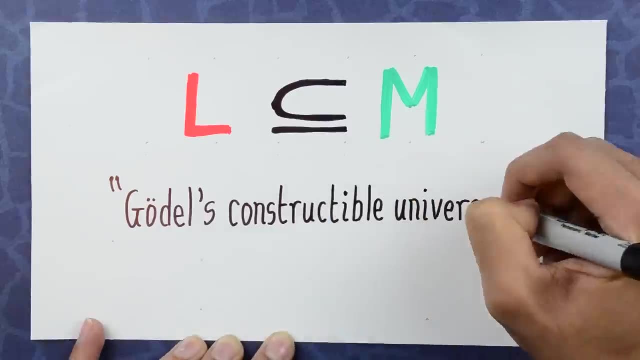 Gettle assumed that we were given a model n ± ZDEF Mikelang when he was M of ZFC. He then constructed a subset L of M called the Gödel-constructible universe, where the continuum hypothesis is true. Then, several years later, Paul Cohen entered the scene. 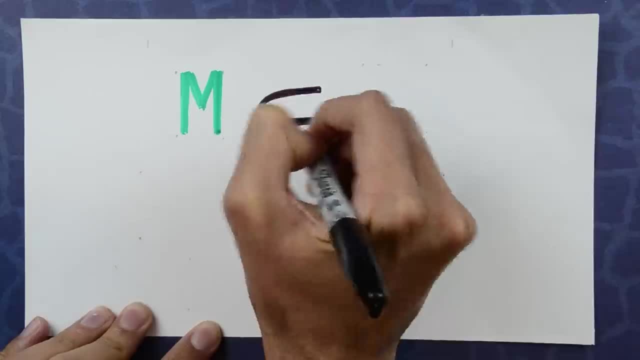 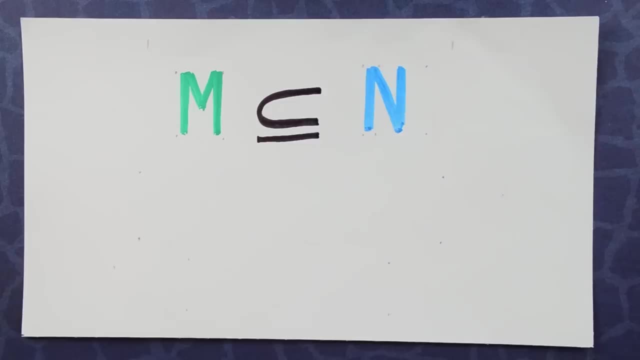 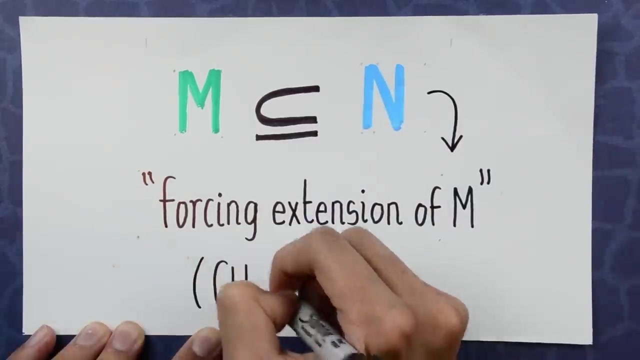 Cohen started with the model M of ZFC and instead of considering a smaller model, he found a way to extend it to a bigger model N containing M. This was later called a forcing extension of M, And in this bigger model N, the continuum hypothesis was false. 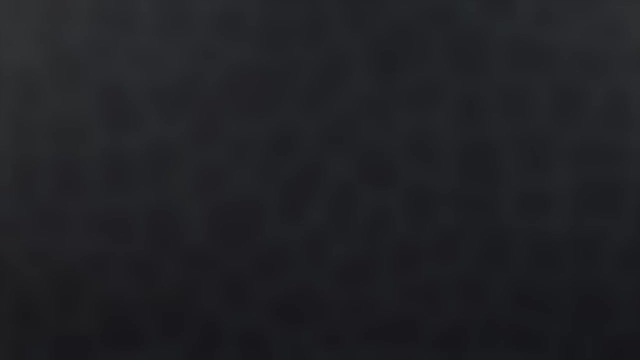 And for this he was awarded the 1966 Fields Medal. Since 1966, people have discovered tons of other statements that were independent of ZFC. The continuum hypothesis is just one of many statements that cannot be decided from the axioms of set theory.